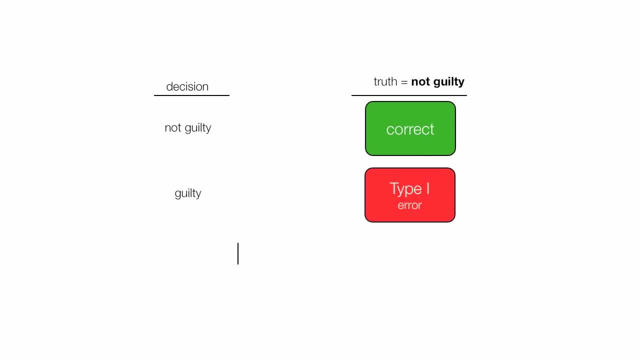 Truth is equal to guilty And then truth is equal to not guilty. The null hypothesis would be something like: we assume the accused is not guilty And the emphasis on not guilty. I'm going to build this table one column at a time. 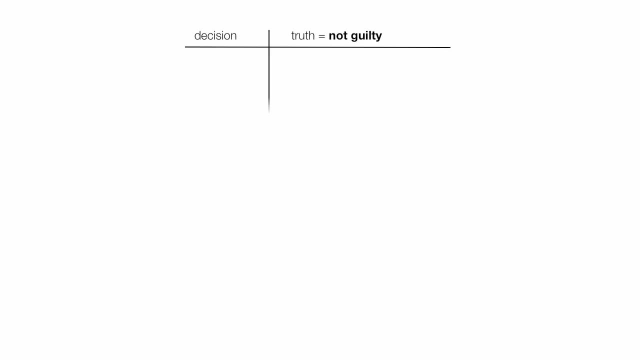 The decision column and the truth column And the decision is either not guilty or guilty. The null hypothesis, the accused is not guilty. We can accept and deny The null hypothesis or we can reject the null hypothesis With an emphasis on not guilty. 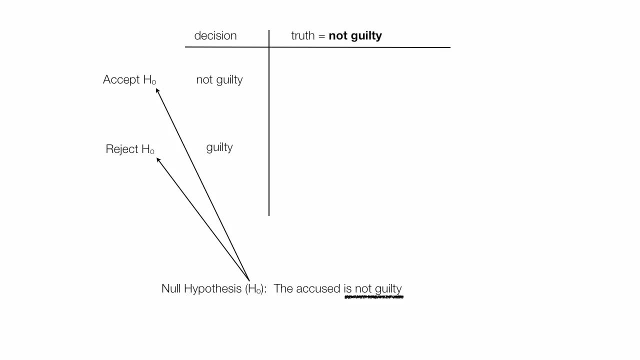 That HO is the symbol or shorthand for null hypothesis. So the first row is we accept the null hypothesis and we say the accused is not guilty, Which turns out to be the reality in this case, And that's good right Now. on the other hand, if we reject the null hypothesis and we say the accused is not guilty, 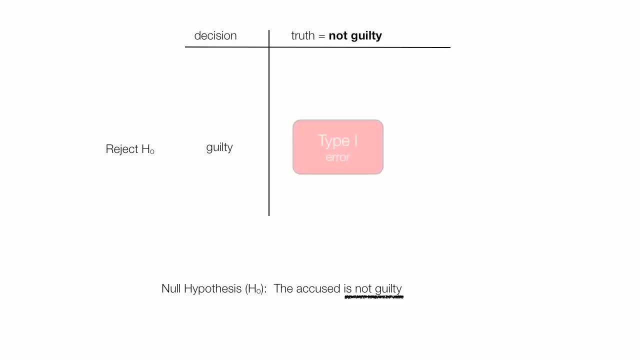 and we reject the null hypothesis and say the defendant is guilty, we commit a type 1 error, alpha and we're finding an innocent person guilty, Which is not very good, It's a bad thing. Remember, in this situation, the correct decision is to accept the null hypothesis. 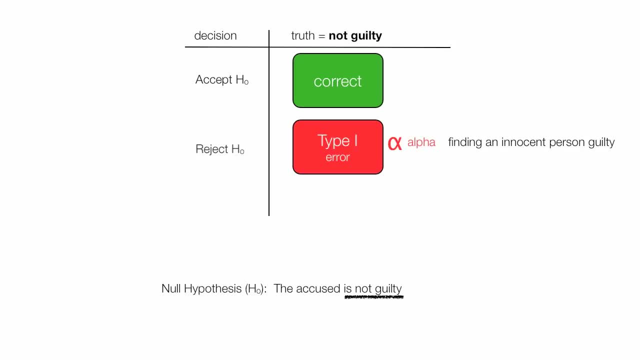 and find the accused not guilty. Accepting the null hypothesis is correct. Rejecting the null hypothesis is wrong. Now, if I change the truth or the reality to guilty, if I find the defendant not guilty when they're guilty, I commit a type 2 error. 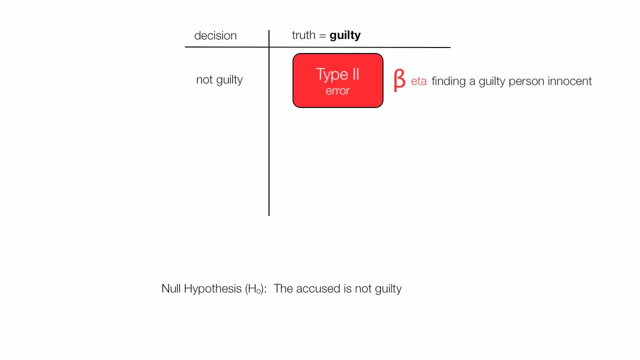 That's called beta- the Greek alphabet beta- and finding a guilty person innocent. On the other hand, if I find the person guilty because they are guilty, that's the correct decision and I reject the null hypothesis. In this case, accepting the null hypothesis is a type 2 error. 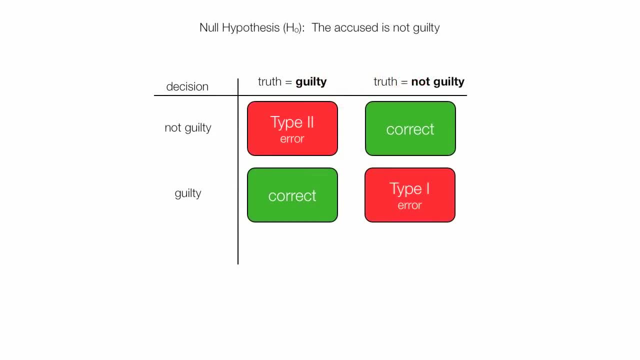 and rejecting it is the correct decision. In hypothesis testing we try to avoid making type 2 or type 1 errors. Typically, type 1 errors are worse than type 2 errors. Putting an innocent person in prison is bad. Now, in this next example, the null hypothesis is animations do not help students improve SAT math scores. 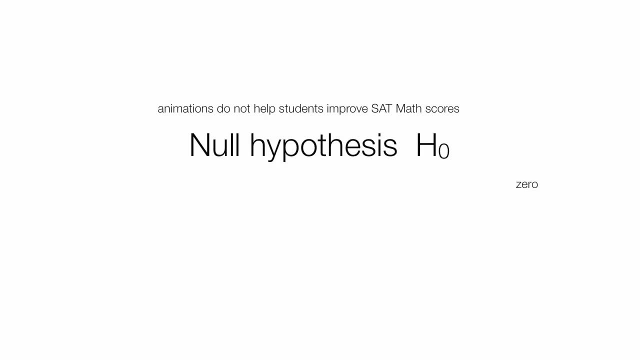 My animations have no impact. Zero effect, None, Nada, Zip, No impact. Animations have no effect, Like a treatment you may be doing may have no effect, and I want to prove beyond a shadow of a doubt that my animations work. 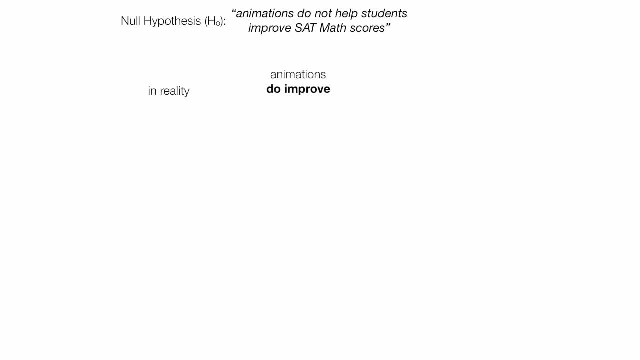 So I make a table. In reality, animations do improve and animations do not improve in columns. Then I also have this column I'm putting in: I can either accept the null hypothesis or reject the null hypothesis. Rejecting the null hypothesis is the correct decision in this case. 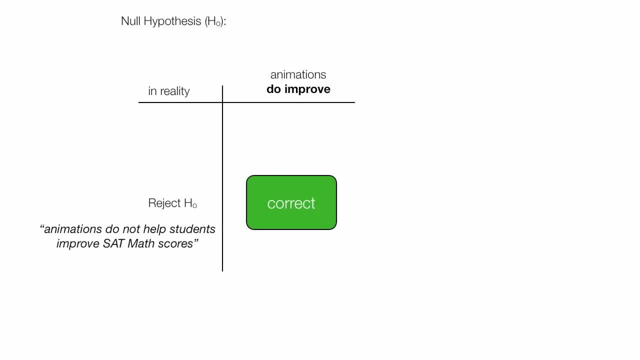 because animations do improve. I'm rejecting the notion, the statement: animations do not help students improve SAT math scores. I'm rejecting this. If, in reality, the animations do not help improve test scores, I would accept the null hypothesis. I say that this statement is correct. 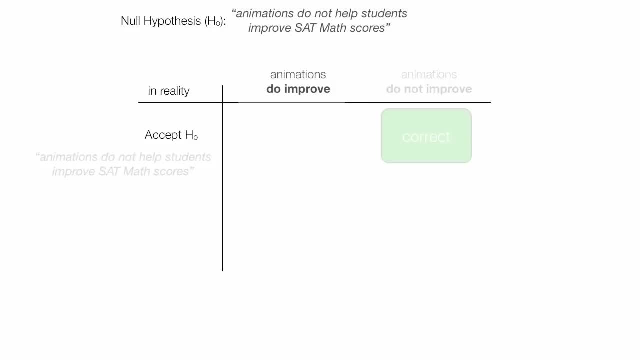 because animations do not help students. If, in reality, animations do improve test scores and I accept the null hypothesis, then I commit a type 2 error Beta. If my animations do not improve test scores and I reject the null hypothesis. 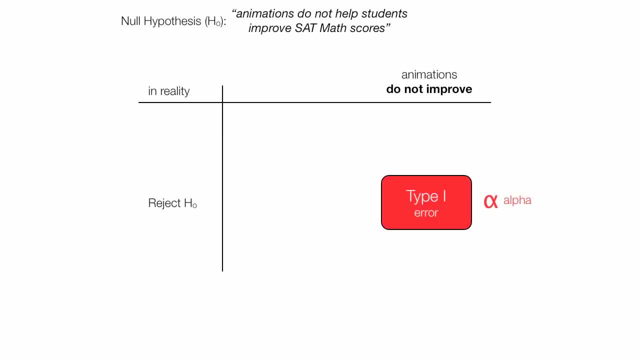 If I reject the null hypothesis, I commit a type one error or alpha. I'm going to build this table again in reality, and the two columns, the three columns actually. If I reject the null hypothesis and animations do improve test scores, I make the correct decision. 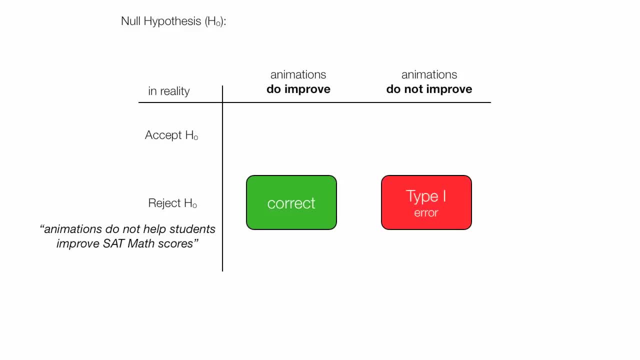 If I reject the null hypothesis and animations do not help students improve SAT math scores, I commit a type one error If I accept the null hypothesis and agree with the statement animations do not help students and animations actually do not help students. that's the correct decision.